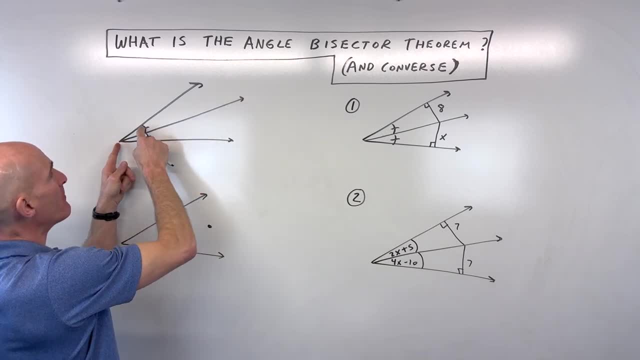 you have this angle here and you draw a ray that bisects, meaning it cuts the angle in half. If you pick a point anywhere along this angle- bisector, let's just say right here- and you measure the perpendicular distance. Now it's important that you always measure the 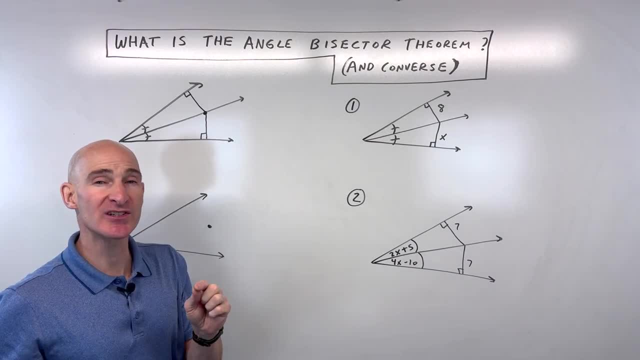 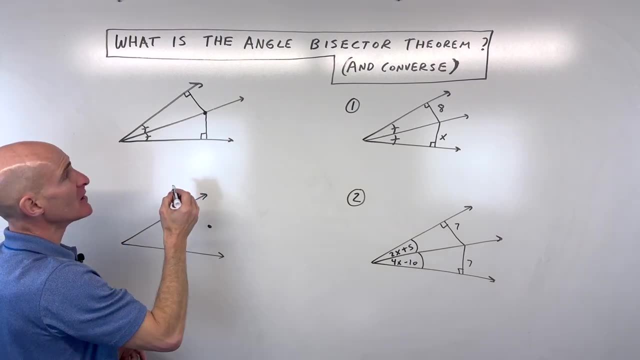 perpendicular distance or the right angle distance, because that's the shortest distance from a point to a line. And what happens is, when you draw that perpendicular distance, these two distances are going to be congruent to one another. Now you might be saying, Mario, 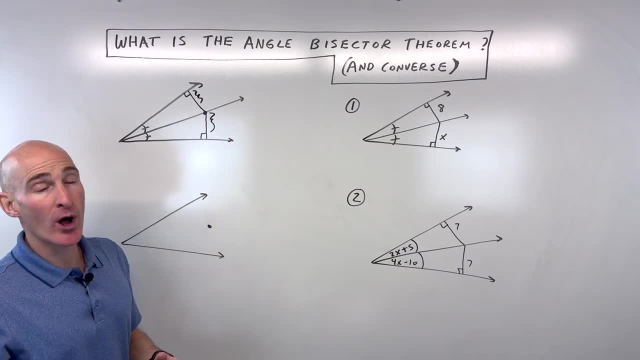 why are these two distances the same? Why does that work? Well, notice that they share this side in between the two triangles by the reflexive property, And you can see that these are both right triangles, and by the angle angle side, angle angle side. 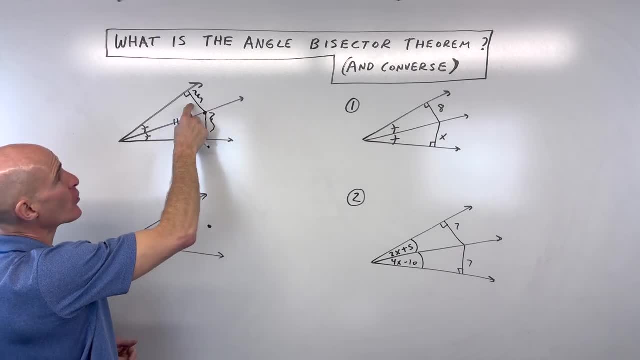 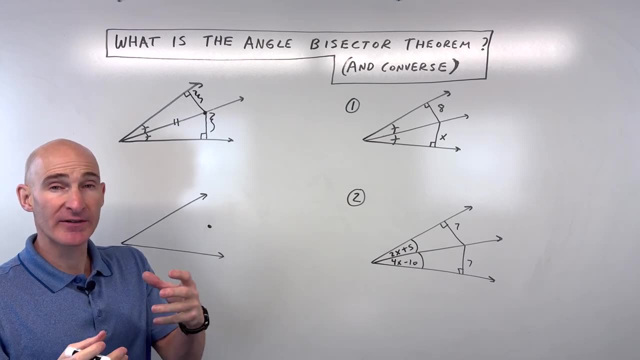 the two triangles are congruent. So therefore, by CPCTC the corresponding parts of congruent triangles will be congruent. So that's why it works is based on congruent triangles. Now, when you look at the converse of the angle bisector theorem, what is that saying? Well, say you have. 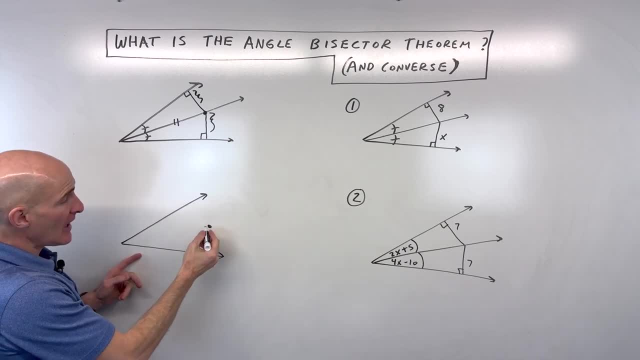 an angle and you pick a point on the interior of this angle and you measure the perpendicular distance to both sides of the angle. If those distances are the same, what do you know about the angle bisector? Well, you can see that the angle bisector is congruent because the 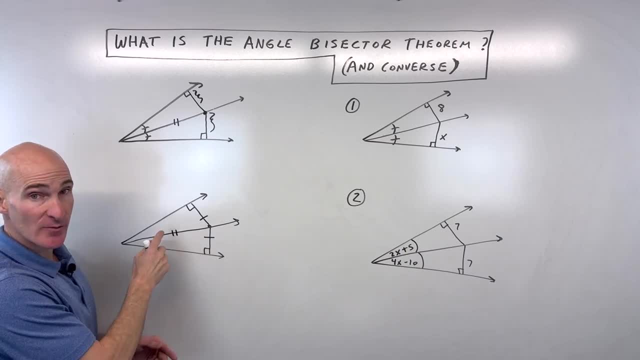 angle bisector is the angle that lies on the angle bisector. Now you can prove this to yourself by using congruent triangles. Again, we notice that this is congruent because it's shared between the two triangles by the reflexive property. They're both right triangles. The hypotenuse is congruent. 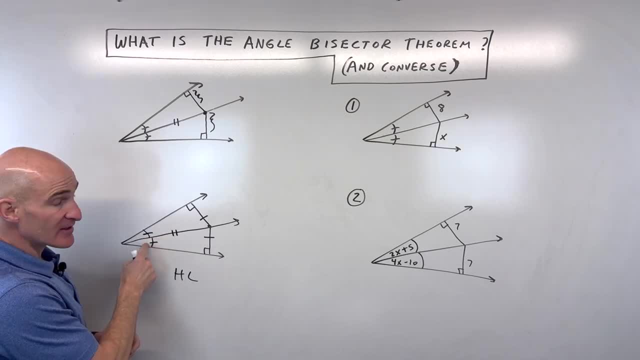 in both triangles and one of the legs is both congruent in both the triangles. So that's the hypotenuse leg theorem And by CPCTC the corresponding parts of congruent triangles, the angle bisector. Okay, so let's go through a couple examples so you can see how this works. 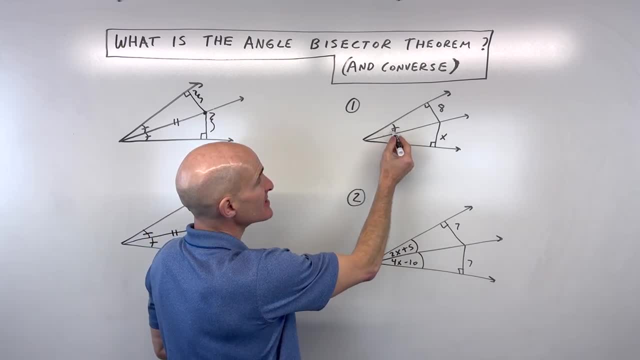 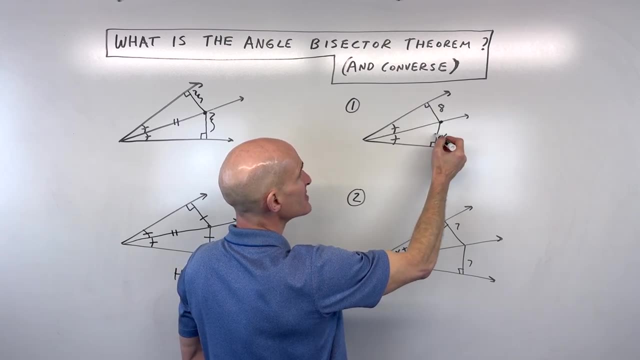 So for number one notice we have, they're giving us that this is an angle bisector. right, because these angles are congruent. So if we have a point here on the angle bisector, what do we know about the distances to the sides of the angle? They must be congruent. So that tells us that x is equal to